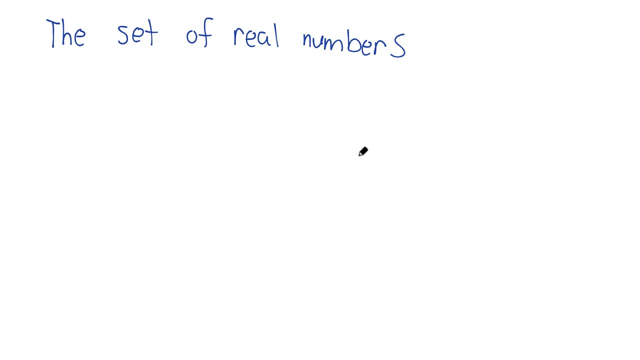 Finally, we are going to start talking about the real numbers. you know the main subject of real analysis. Now this video. maybe it's a little bit of a cop out because we're not going to actually construct the real numbers like you would in some courses. This course that I'm making is really just designed as an intro course and trying to get you off the ground and get you started and dealing with this stuff as quickly as possible. So we're just going to sort of just take this for granted. This won't be 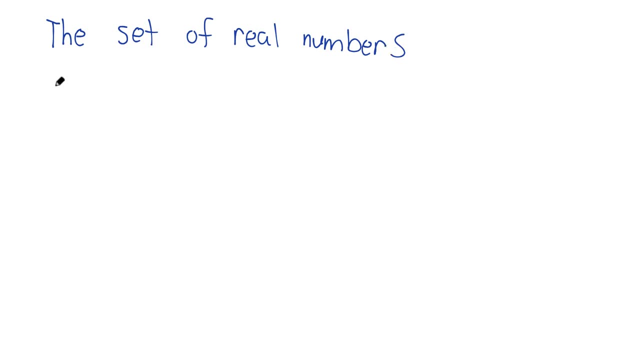 what you do in every class, But for us we are. we're finally going to just say the set of real numbers. This is the topic, And you can call this a theorem, if you like. Theorem, There exists in fact a unique one, And so sometimes, if you've seen the, there exists, sometimes we put a exclamation point. So this means there exists a unique, there's only one of them. there exists a unique ordered field. So we talked about 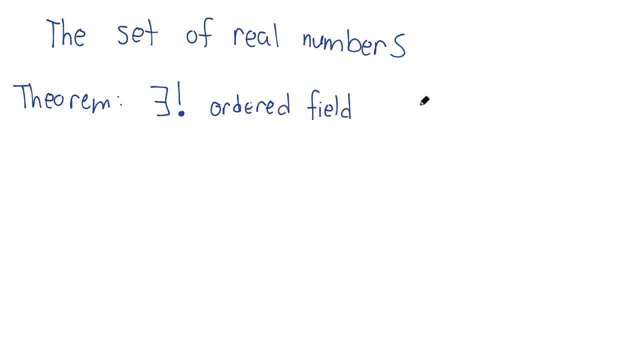 fields and we talked about ordered fields And this ordered field. it has the least upper bound property, Also known as the completeness property. We talked about that in a video as well. With the completeness property, There exists a unique ordered field with the completeness property, such that the field Q is a subset. This is the script R that we'll be using. 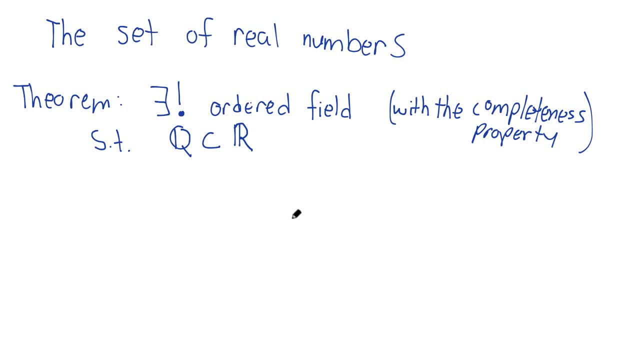 to describe the real numbers. you may have seen it before, but this is the theorem: there exists a unique ordered field with the completeness property having q as a subset, very, very powerful. i'm just going to ask you in this video to accept this, but you're welcome to do your own. 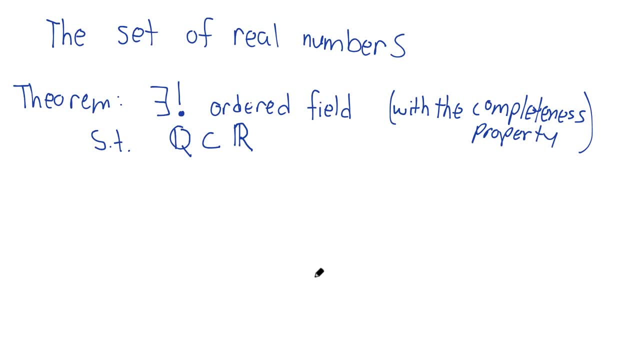 investigation. if you'd like to see proofs of this, from now on we'll be able to use this fact and anytime you see this special character r, know that we're talking about the set of real numbers. 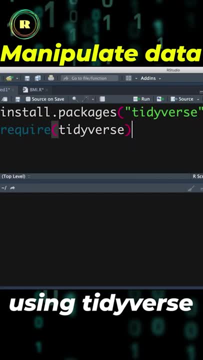 I've already installed the tidyverse package. You only ever have to do that once. Once it's been done once, you never do it again. But every time you want to use that package in a new session you have to say either require or library.